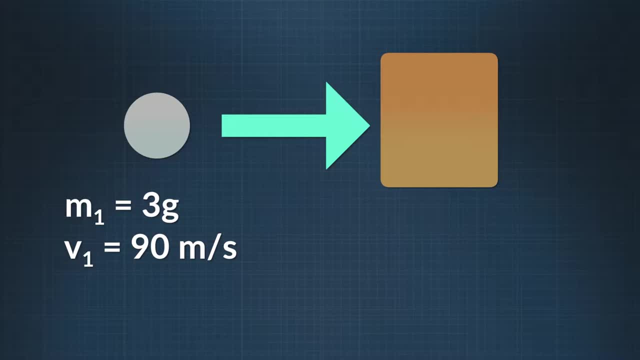 So it has momentum. The total momentum of our system before the collision is the momentum of the paintball, because the barrier, which has a mass of 9 kilograms, is initially at rest and has no momentum. Remember, an object's momentum is equal to its mass, times its velocity. 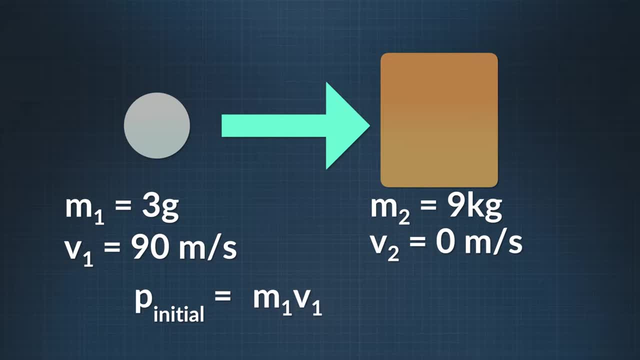 We convert the mass of the paintball from grams to kilograms and get 0.003 kilograms. We then multiply this times the 90 meters, Times the 90 meters per second velocity and end up with a momentum of 0.270 kilograms meters per second. 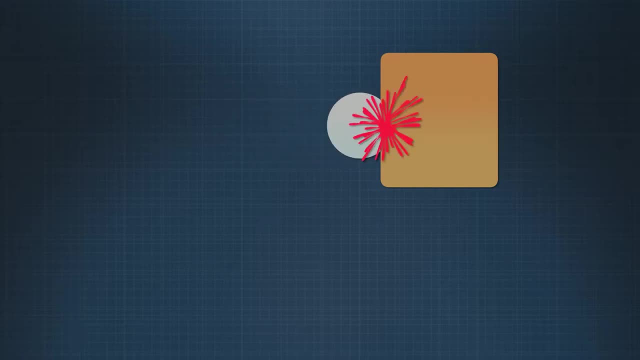 When the paintball and the barrier collide, the momentum in the system must be the same both before and after the collision happens. The paintball and the barrier are moving together after the collision, so we add their masses to get the total mass of the system. 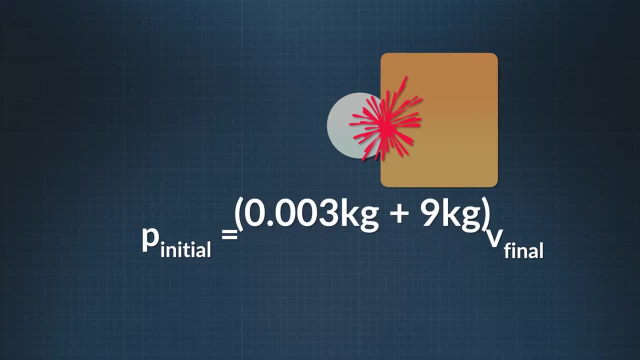 which is the mass of the paintball- 0.003 kilograms, plus the mass of the barrier: 9 kilograms, for a total of 9.003 kilograms. Then we set the momentum of our system: 0.270 kilograms meters per second. 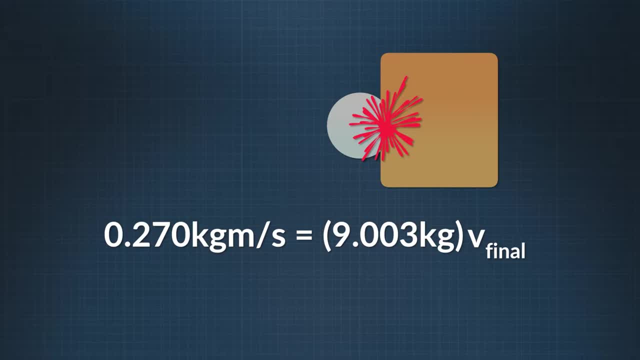 equal to the combined mass of the paintball and the barrier: 9.003 kilograms times the final velocity of the paintball and barrier together. In order to solve for the final velocity, we must divide the momentum by the total mass and we end up with a final velocity of 0.03 meters per second. 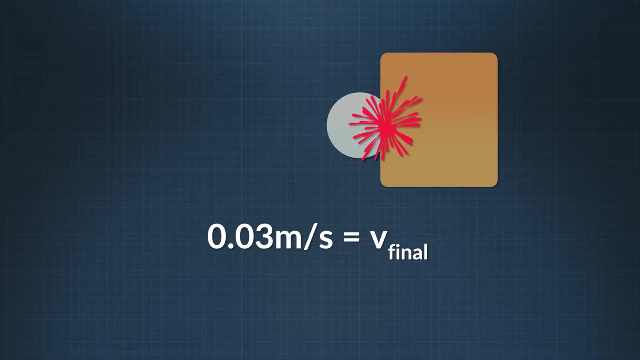 Keep in mind that this velocity only holds for the instant after the collision. Eventually, both the paintball and the barrier slow down until they're at rest at 0 meters per second. The second type of collision, as we mentioned, is an elastic collision. 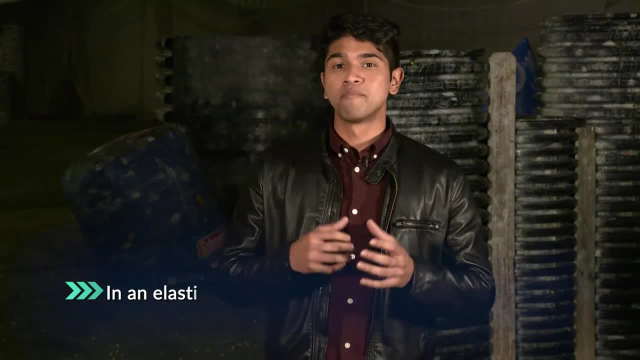 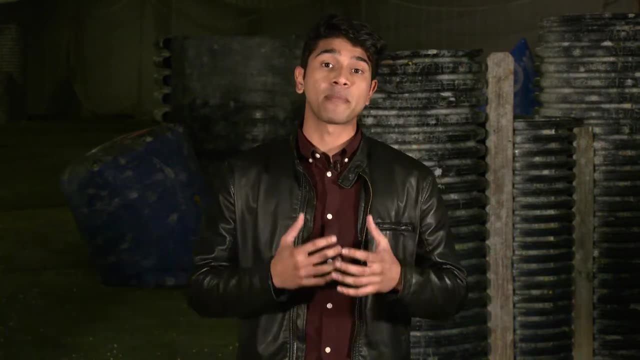 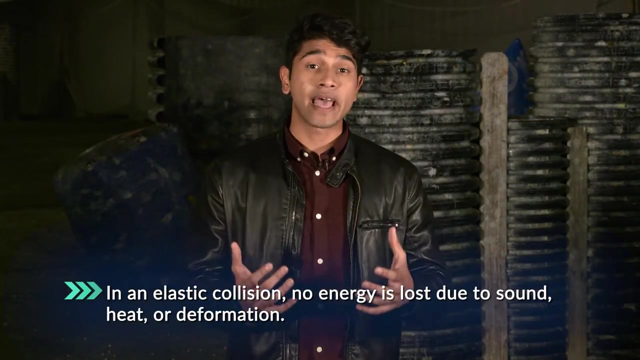 That's when two objects bounce apart. when they collide, Momentum and kinetic energy are both conserved, meaning the amount of momentum and kinetic energy in the system is the same after the collision as it was before the collision. Also, in an elastic collision, no energy is lost due to sound, heat or deformation. 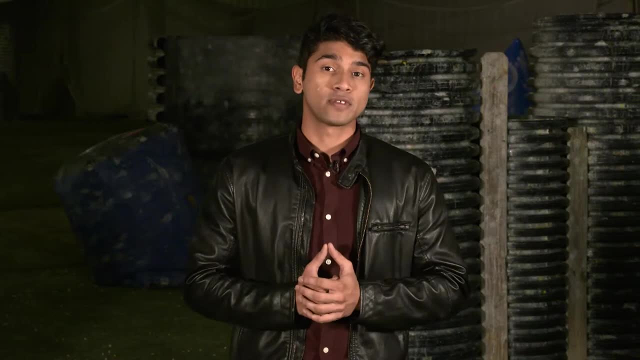 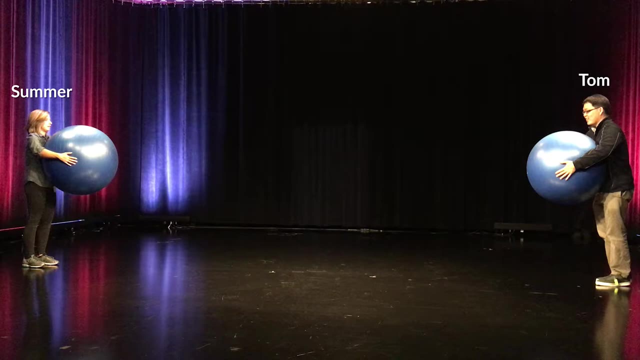 which is a change in the shape or size of an object due to force, In other words, dents, dings and the like. Let's do a problem using an elastic collision, with the help of Summer and Tom and two rubber exercise balls. 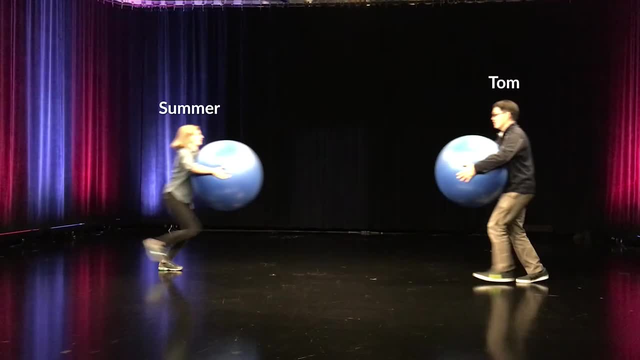 Okay, let's stop the video for a second while I give you some information about what's happening. Tom has a mass of 75 kilograms and is running at a velocity of negative 1 meter per second holding an exercise ball. Summer has a mass of 50 kilograms and is running at a velocity of 4 meters per second. 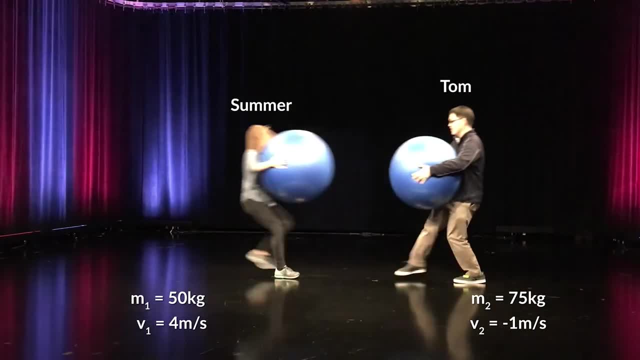 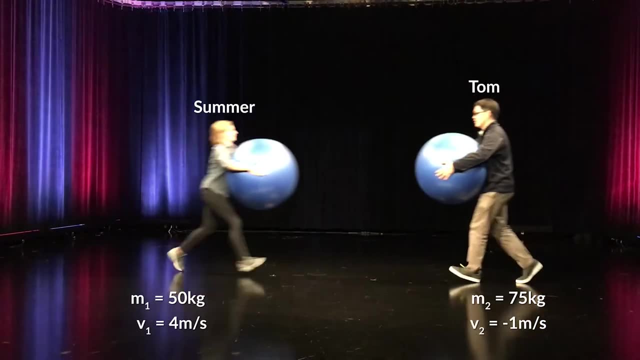 also holding an exercise ball. Okay, play the video. Now that's an elastic collision- if I ever saw one. What happens when they bounce off of each other? If 50 kilograms Summer bounces backward with a velocity of negative 2 meters per second? 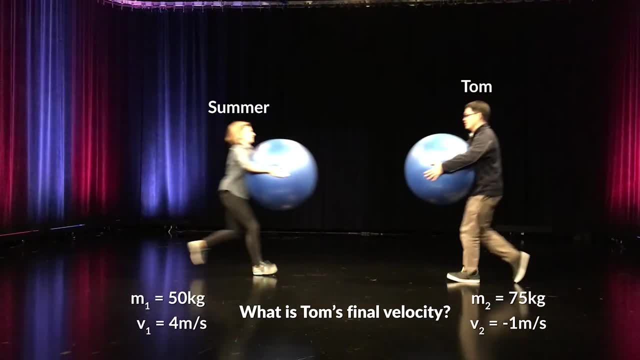 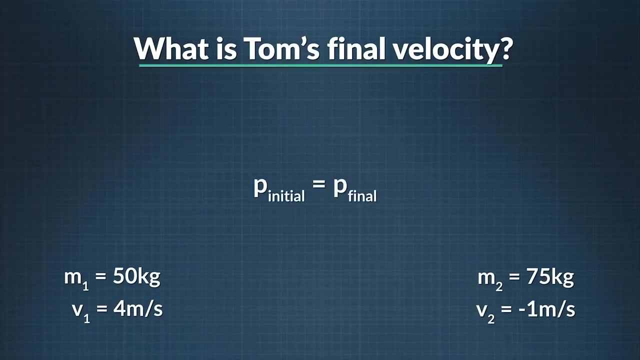 what is Tom's final velocity? Remember that momentum is conserved in all collisions, so we always start with that which is: p sub i equals p sub f. Now let's determine the initial momentum by adding up the momentum of each person. 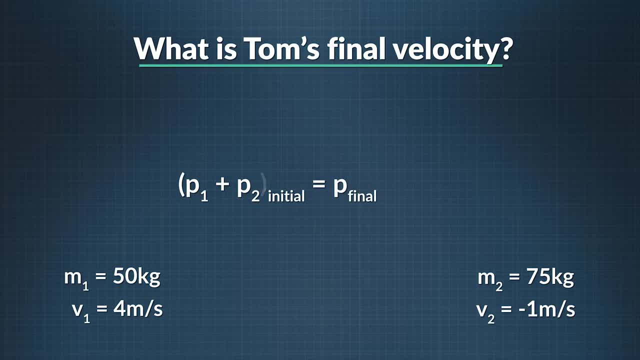 Plug in the equation for an object's momentum which, remember, is its mass times its velocity. We do this for Summer and for Tom. Summer's mass is 50 kilograms and her velocity is 4 meters per second. Tom's mass is 75 kilograms. 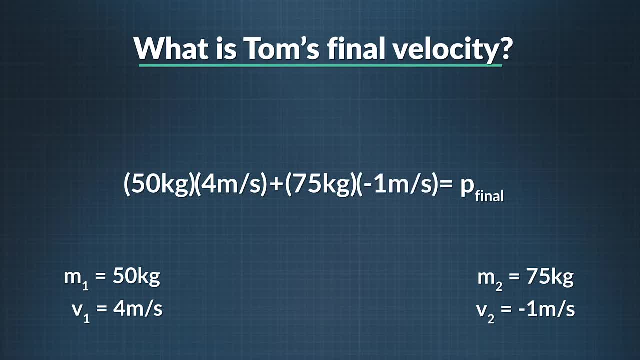 His velocity is negative 1 meter per second. We make his velocity negative because he moves in the opposite direction of Summer. Multiply 50 kilograms times 4 meters per second and add it to 75 kilograms times negative 1 meters per second. 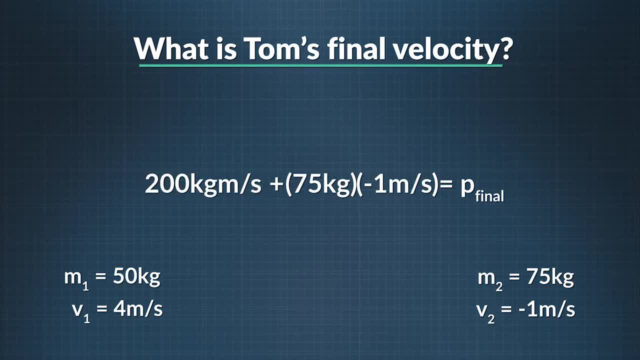 Summer's initial momentum is 200 kilograms meters per second and Tom's initial momentum is negative: 75 kilograms meters per second. When we combine those two together, we get a total momentum of the system of 125 kilograms meters per second before the collision. 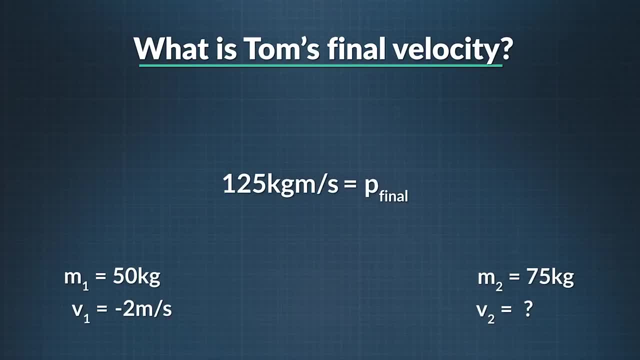 Our initial and final momentum must be the same: 125 kilograms meters per second. So let's solve for the final momentum in the system. for each of the two people We plug in the values that we know, The total momentum is equal to 125 kilograms meters per second.